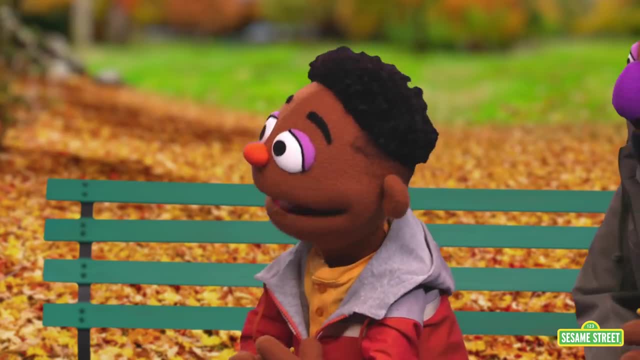 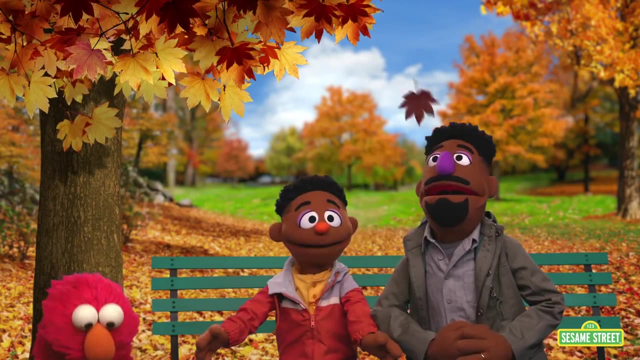 Hi, What are you two doing? Dad and I are taking a break from our nature walk, Yep, and we stop for a moment to enjoy the colorful leaves. Oh yeah, Oh look, Elmo, the leaves are falling, Yeah. 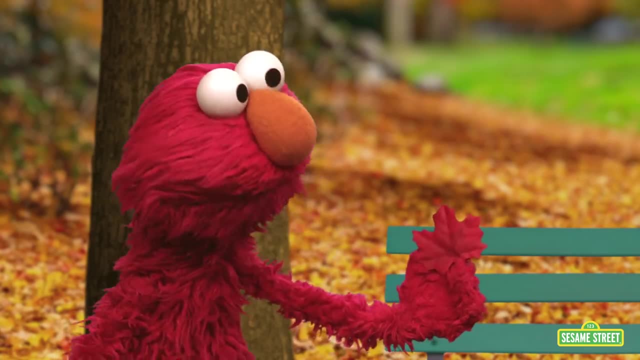 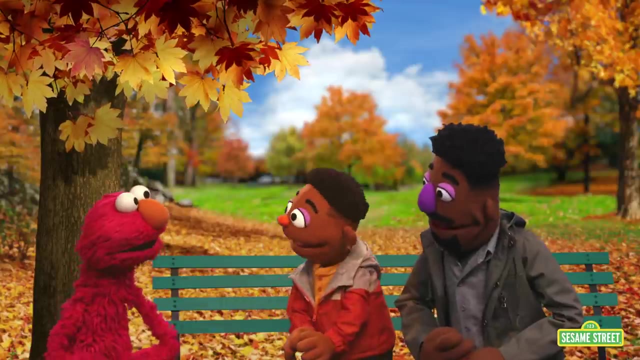 Look, look, This leaf is red like Elmo's fur, Oh, oh, oh. And this leaf is brown like Russ's skin. Good observation, Elmo. Oh, thank you. Oh, Elmo has a question. Oh, oh, what is it, Elmo? 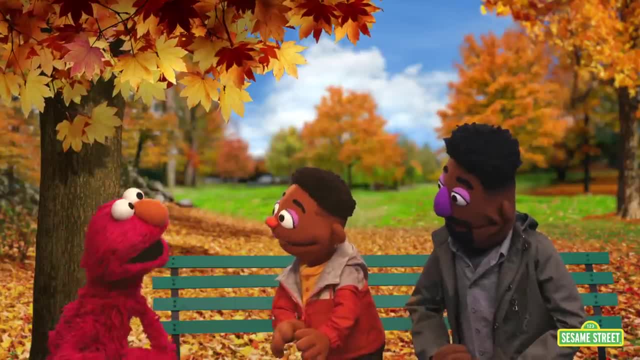 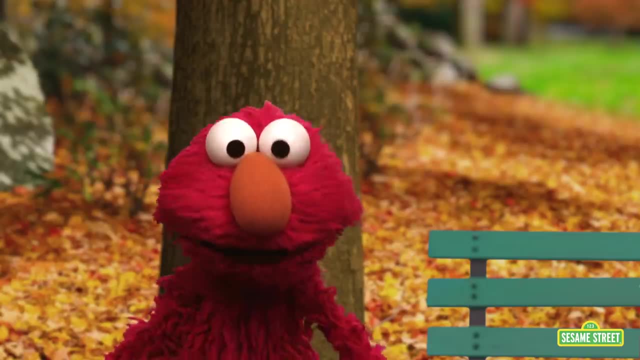 Well, Elmo wants to know why Russ's skin is brown. Oh, I know why, Elmo. My mom and dad told me It's because of melanin. Right, Dad? That's right, Melanin. Oh, oh, what's that? 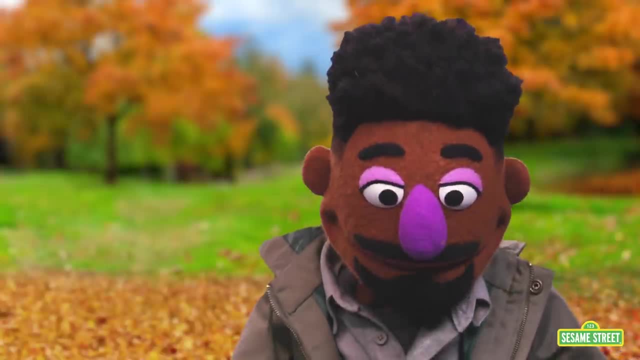 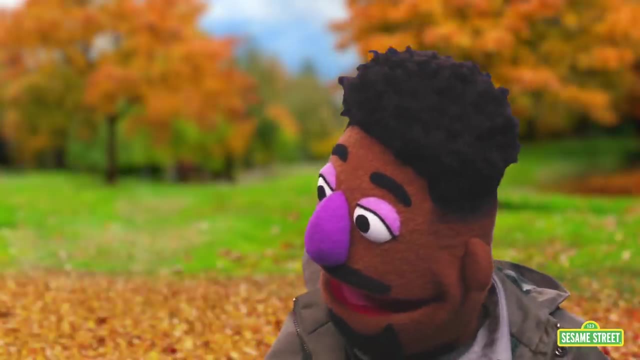 Well, melanin is something that we each have inside our bodies that make the outside of our bodies the skin color that it is. It also gives us our eye and our hair color, Oh, and our fur color. Yes, that's right. 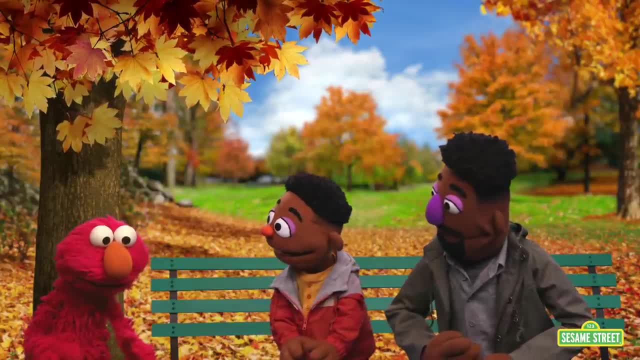 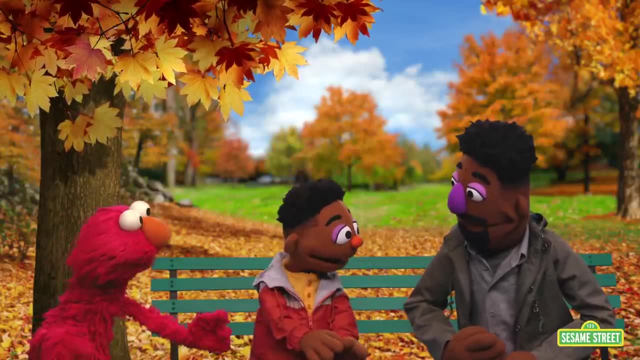 Exactly, Elmo. Oh, but if we all have melanin, why are we different colors? Like, why is Mr Elijah's skin a darker brown than Russ's skin? Oh, that's a good question, Elmo. Well, it's because the more melanin you have. 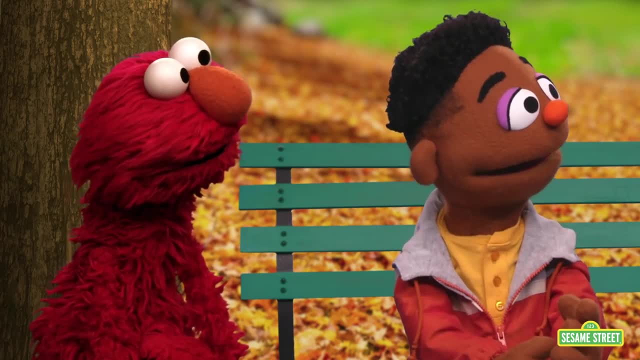 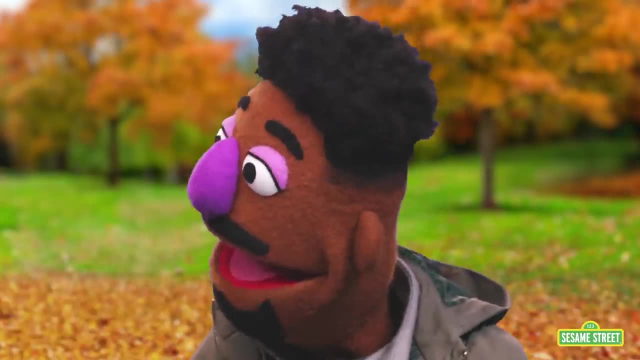 the darker your skin looks. Oh, The color of our skin is an important thing, because our skin is an important part of who we are, But we should all know that it's okay that we all look different in so very many ways. Oh well, Elmo's fur is red and soft. 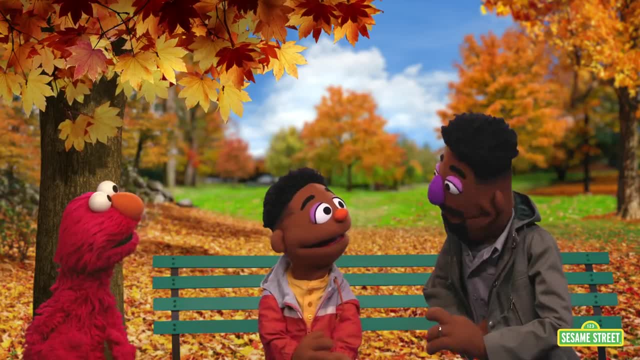 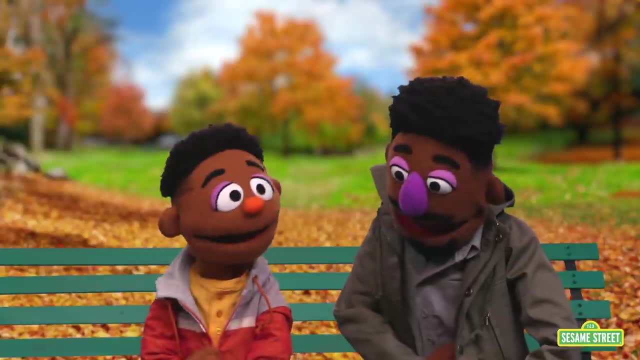 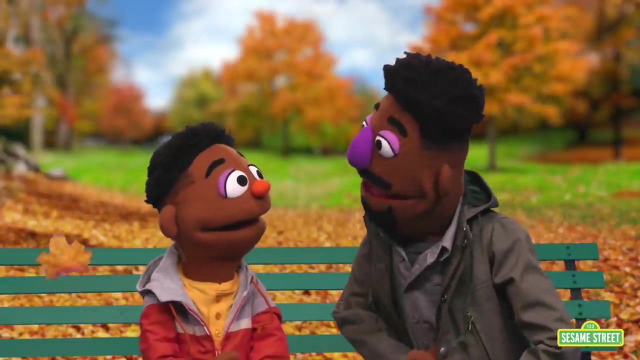 Oh, and my hair is black and curly. Things on the outside like our skin color, our hair texture, our noses, our mouths and eyes make us who we are. Many people call this race, But even though we look different, 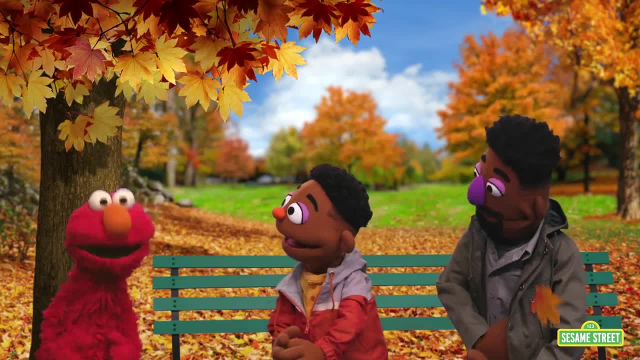 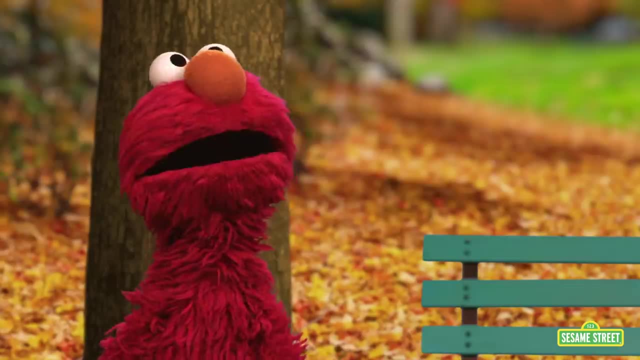 we're all part of the human race, Isn't it cool? Elmo, Very cool. Huh, Look at the leaves. What do you two see? Elmo sees leaves that are all different colors, And the different colors look really cool together.